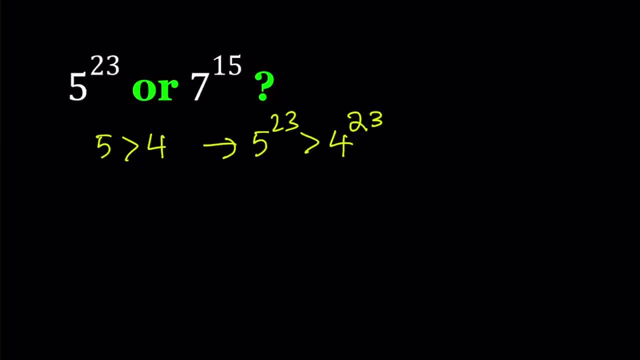 4 to the power 23.. Now 4,. the reason why I said, okay, we're going to use powers of 2 is because 5 is close to 4 and 4 is a power of 2.. And now we can write 4 as 2 squared. 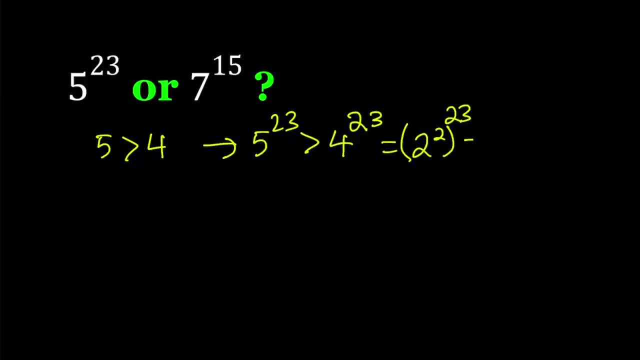 and then it's raised to the power 23. And now, by power of power, we get 2 to the power 46. because we're supposed to multiply the exponents. So we got from here. we get that 5 to the power 23. 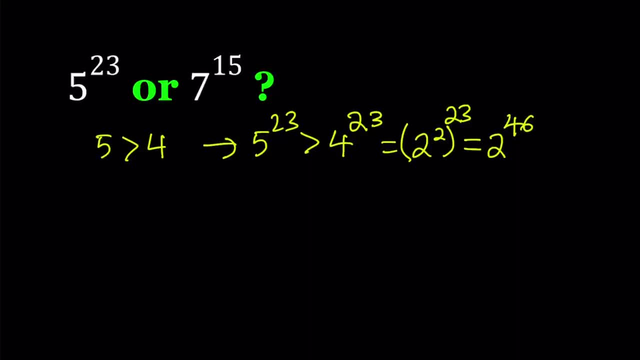 is greater than 2 to the power 46. Let's go ahead and write that down. as a result, 5 to the power 23 is greater than 2 to the power 46. Awesome, Now let's go ahead and do something for the 7.. 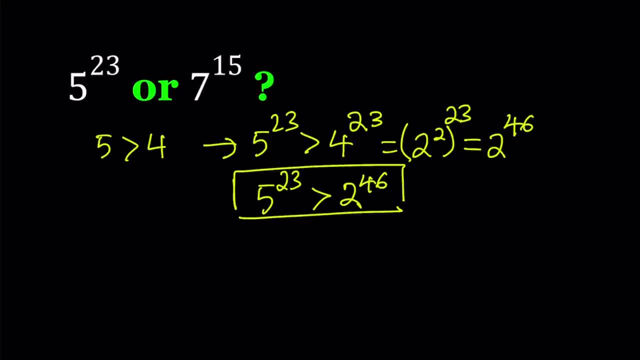 Now, 7 is also close to a power of 2 because it's less than 8.. In other words, 8 is greater than 7.. Therefore, 8 to the power 15 is greater than 7 to the power 15.. 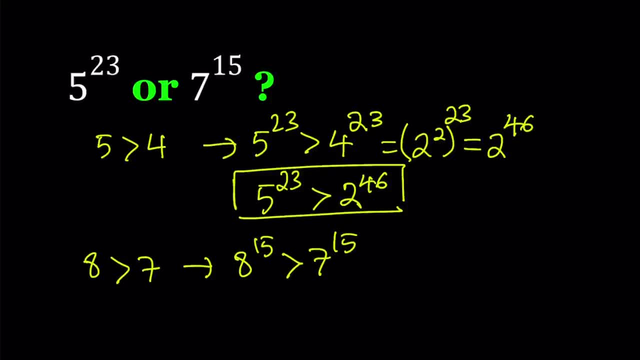 Right, And we do know that 8 to the power 15 is 2 to the power, 3 to the power 15.. Therefore, 8 to the power 15 can be written as 2 to the power 45, because 3 times 15 is 45.. 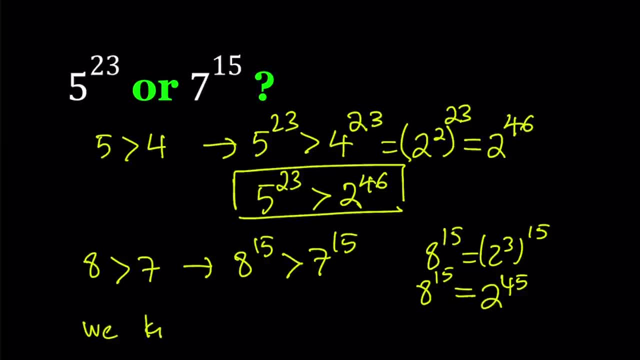 And we also know that. We know that. We know that 2 to the power of 46 is greater than 2 to the power of 45.. Awesome, right, Okay, cool. Why did I compare 2 to the power of 46 to 2 to the power of 45?? 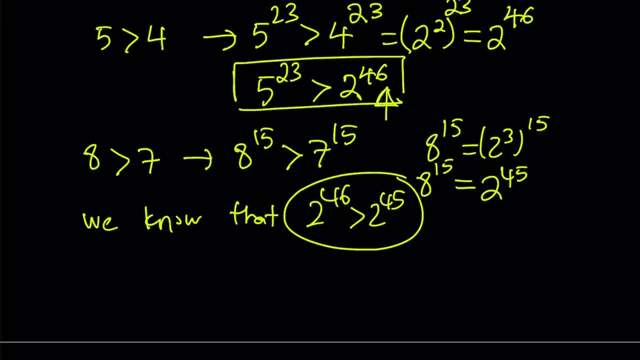 Because now, here we have 2 to the power of 46, and we do know that 8 to the power of 15 is equal to 2 to the power of 45. So let's go ahead and put it all together and arrive at the conclusion. 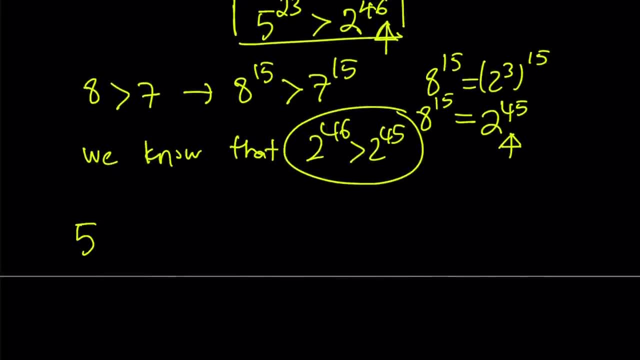 Great. So now we have: 5 to the power of 23 is greater than 4 to the power of 23.. As you know, 4 to the power of 23 can be written as 2 to the power of 46.. 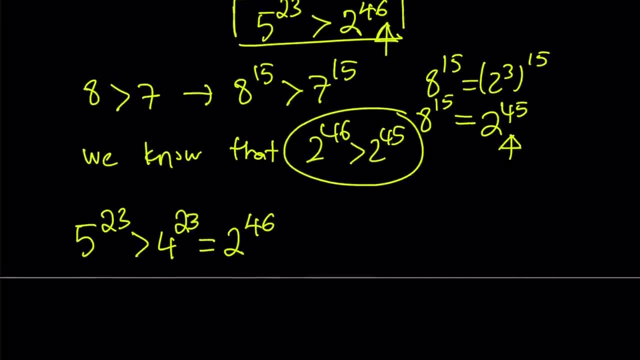 We just established that right up there right, And 2 to the power of 46 is clearly greater than 2 to the power of 45, which is the same thing as 8 to the power of 15, because 8 can be written as 2 to the third power. 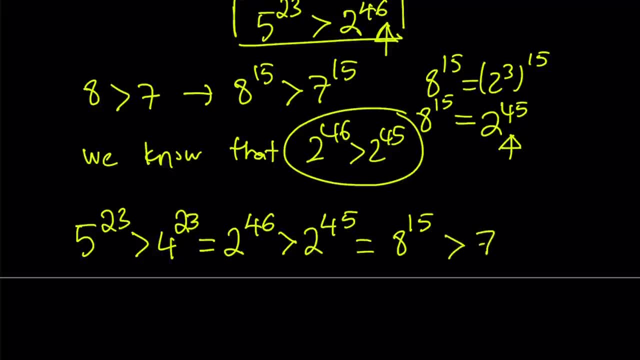 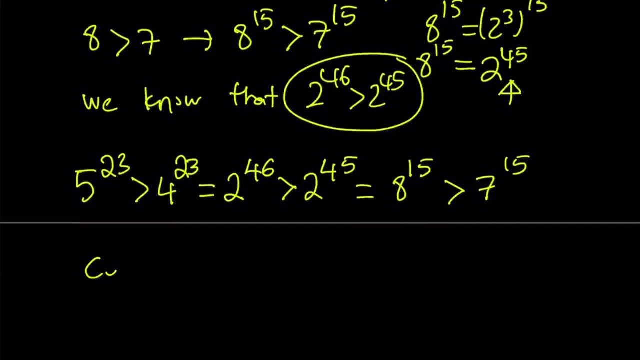 And, obviously, 8 to the power of 15 is greater than 7 to the power of 15.. 7 to the power of 15.. Using all these inequalities and equations, we arrive at the conclusion. The conclusion is: 5 to the power of 23 is greater than 7 to the power of 15.. 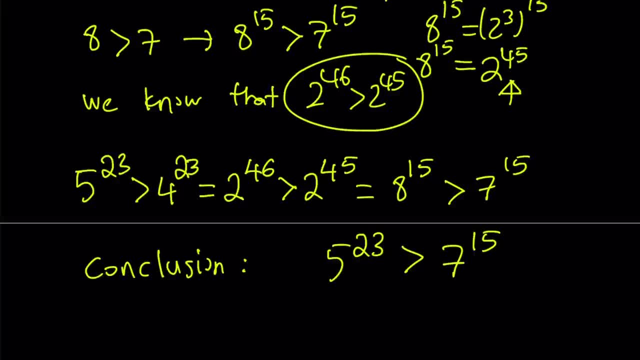 Awesome. So 5 to the power of 23 wins, That's the greater number. You know, a lot of times people say: if you have a situation where we compare, you know two exponential numbers. usually the one with the smaller exponent is the larger one. 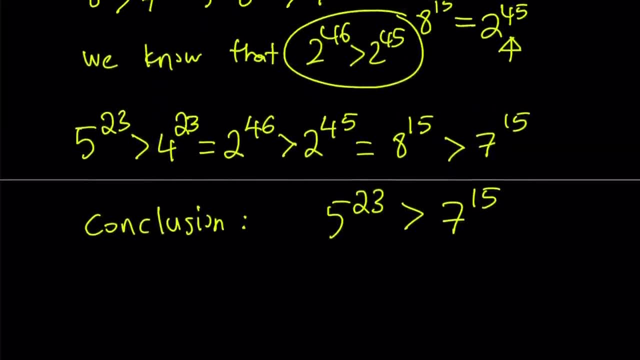 Well, that depends. That depends on the numbers. In this case, the one with the larger exponent wins, And it may, you know, differ from case to case. But I just want to bring up a question. It's going to be like open-ended. 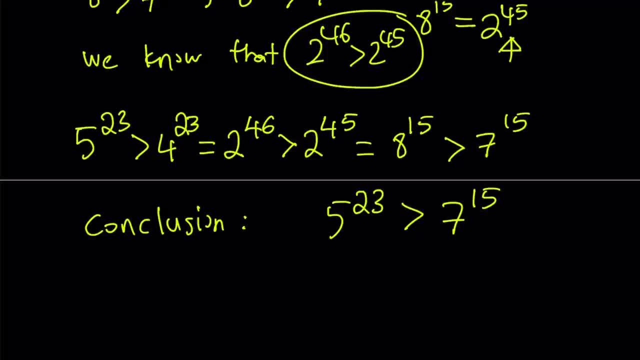 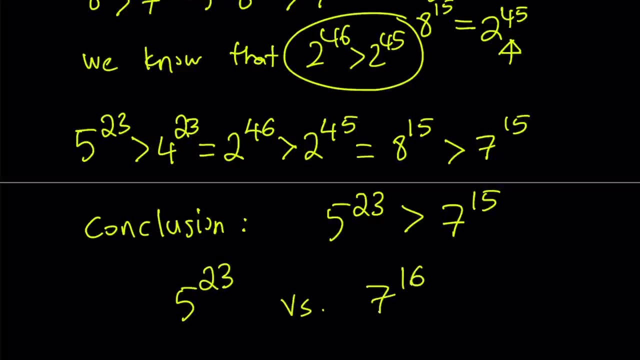 I'm not going to answer it, but I want you to think about it. How about if we had to compare 5 to the power of 23 versus 7 to the power of 16? Would the inequality still hold, or 7 to the power of 16 would be larger? 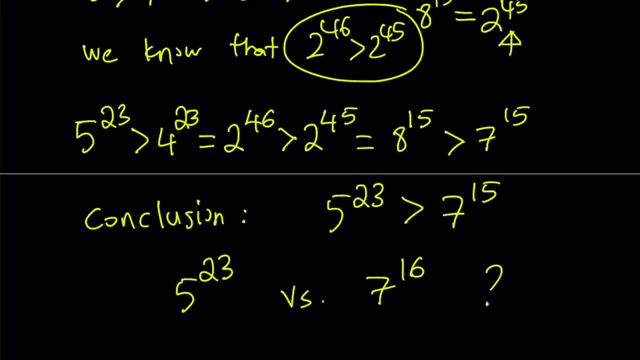 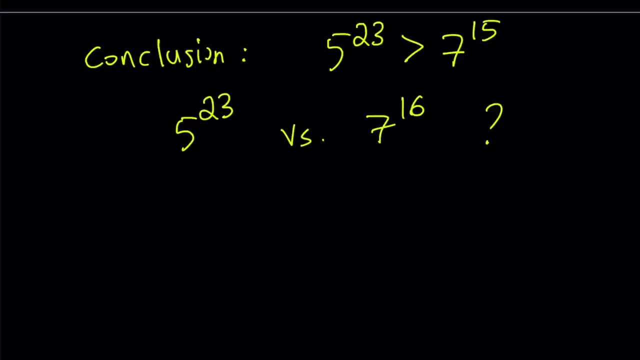 Can we find out? Is there a way to do it? So I just want you to think about this. I want to leave it as an open-ended question, And if you give me some ideas, that would be great. Anyways, let's talk about numerical values and we're going to conclude. 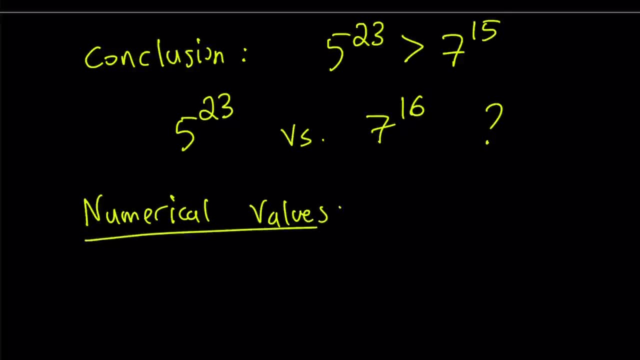 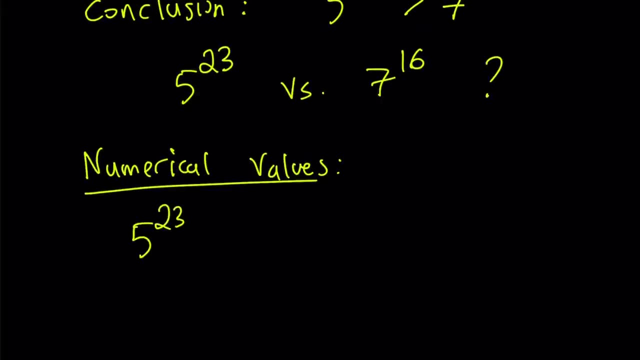 So these numbers are actually very much apart. They're not really close. That's why I wanted to bring up these two numbers for your attention. But if you evaluate them, approximately 5 to the power of 23 is going to be 1.19 times 10 to the power of 16.. 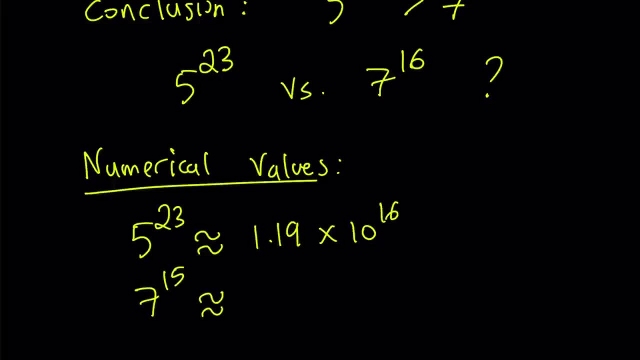 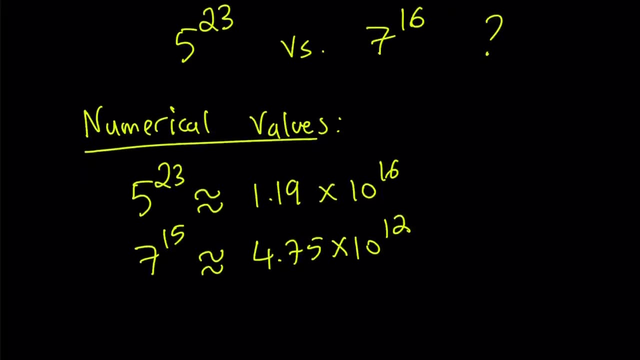 And 7 to the power of 15 is going to be about 4.75 times 10 to the power of 12.. Obviously they are very different, And does that tell you how to compare these numbers? Okay, I already gave the answer for this open-ended question. 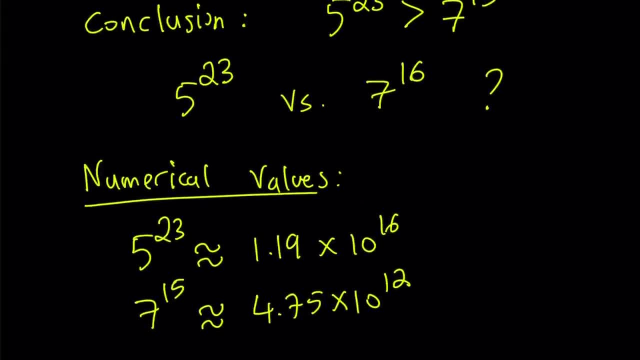 But I guess my question is: how can you prove that one is larger than the other without using the calculator? So ignore the numerical values that I gave you and just think about this problem. And this brings us to the end of this video. Well, thank you for watching. 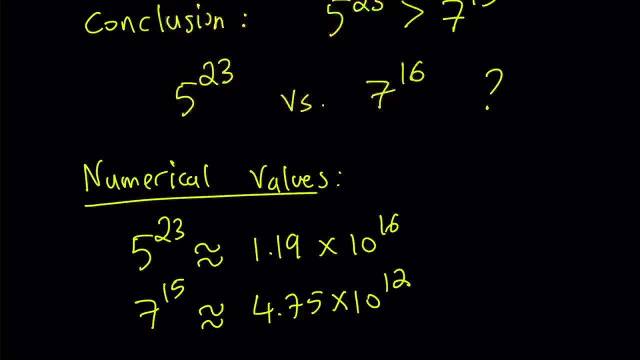 I hope you enjoyed it. Please let me know. Don't forget to comment, like and subscribe. I'll see you tomorrow with another video. Until then, be safe, take care and bye-bye.